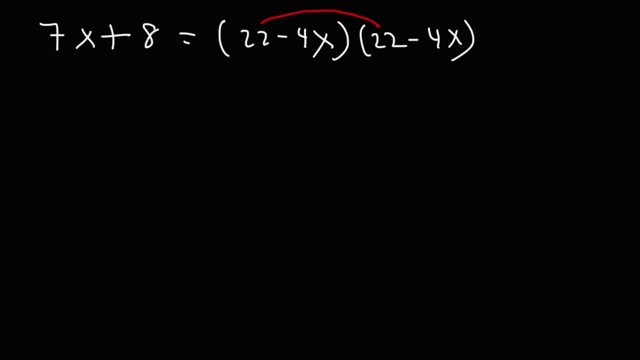 So it's a four. Next, we're going to multiply 22 by 22.. And that is equal to 484.. Next we're going to multiply 22 by negative 4x, So that's negative 88x, And then negative 4x times. 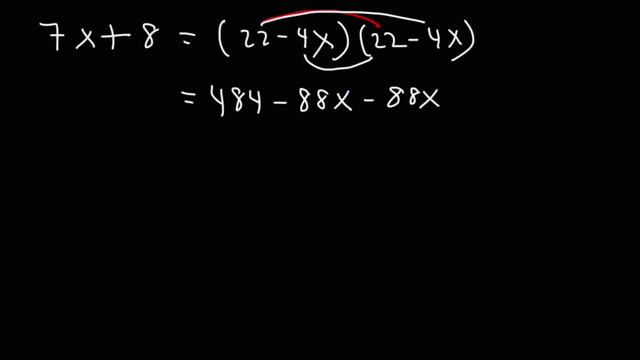 22.. That's going to be the same. And then finally, negative 4x times negative 4x, which is positive, 16x squared. Now let's combine like terms. So we're going to have 16x squared, negative 88 minus 88.. That's. 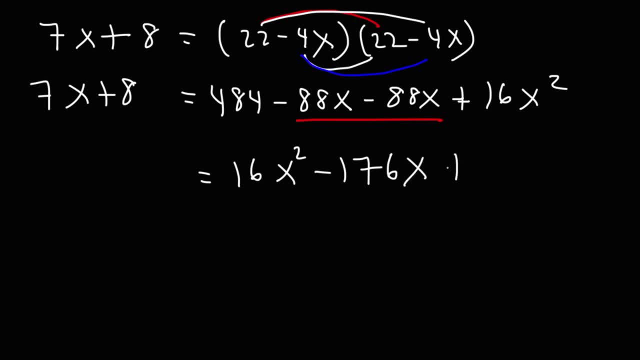 negative 176x And then plus 44. Now we have a quadratic equation on the right side. So what we're going to do is we're going to take everything from the left side, move it to the right side. We can do this in any way we want. We can do this in any way we want. We can do this in any way we want. 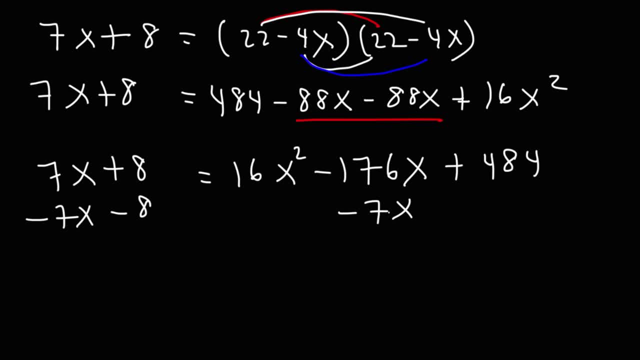 We can do this by subtracting both sides by 7x and by 8.. So we're not going to have anything left over on the left side. On the right side we're going to have 16x squared minus 183x, And then 484 minus 8.. That's positive 476.. 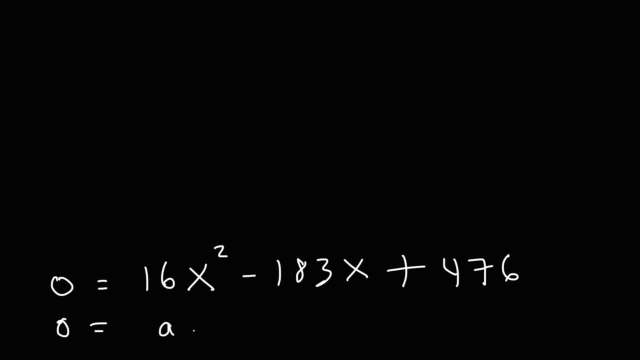 Now, at this point we could use the quadratic formula, which is in the form: ax squared plus bx plus c. So we can clearly see that a is 16, b is negative 183, and c is 476.. So the formula is: x is equal to negative b plus or minus the square root of b squared minus 4ac, divided by 2a. 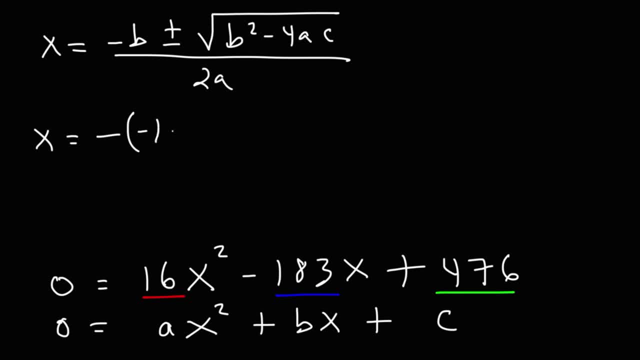 So it's negative. and then times b, which is negative, 183.. b squared, that's negative 183 squared. And then minus 4 times a: a is 16, and c is 476, divided by 2a, or 2 times 16.. 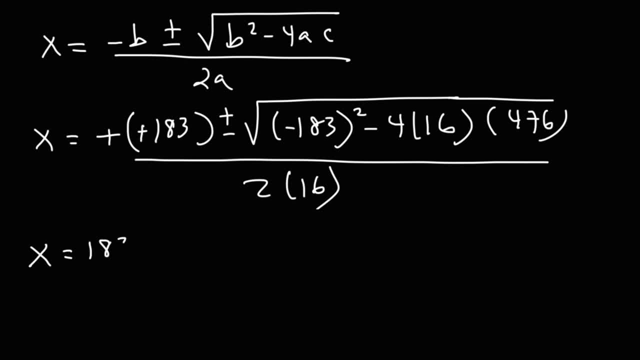 So these two negative signs will cancel giving us positive 183.. 183 squared, that's going to be 33,489.. And then minus 4 times 16, times 476,, that's 30,464.. And then 2 times 16 is 32.. 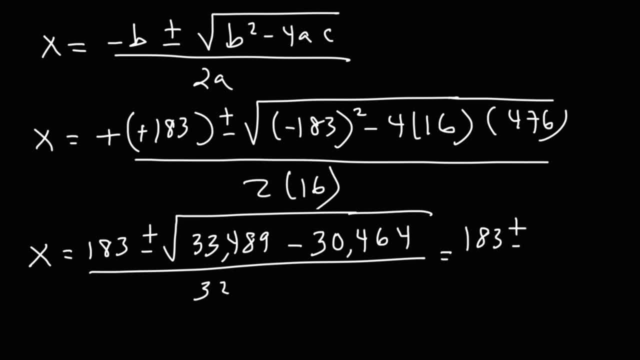 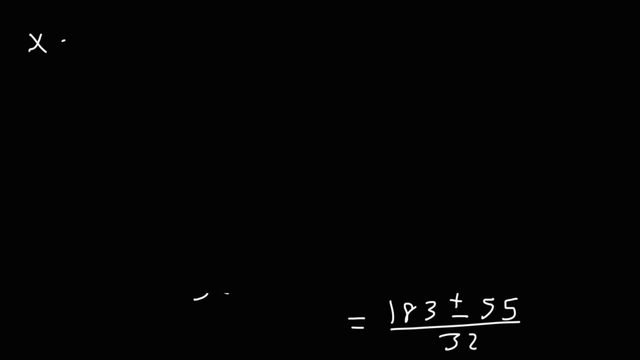 33,489 minus 30,464, that's 3,025.. The square root of 3,025 is 55.. So this will give us potentially two answers. The first one is going to be 183 plus 55, divided by 32.. 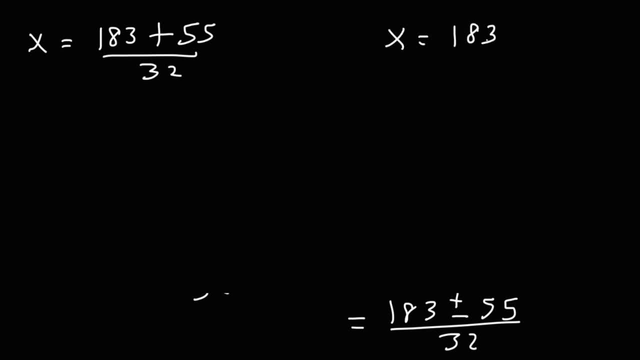 And for the second one, we have 183 minus 55, divided by 32.. 183 plus 55,, that's 238.. And 238 divided by 32.. You can reduce that to 119 over 68. That's 16, if you divide both numbers by 2.. 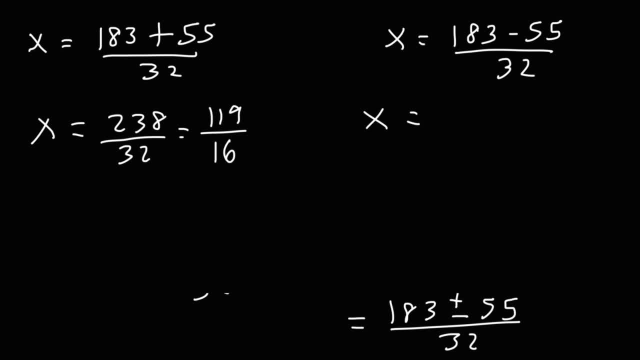 For the next one, 183 minus 55 is 128, and 128 divided by 32 is 4.. So we have two potential answers: x is equal to 4, and x is equal to 119 over 16, which? 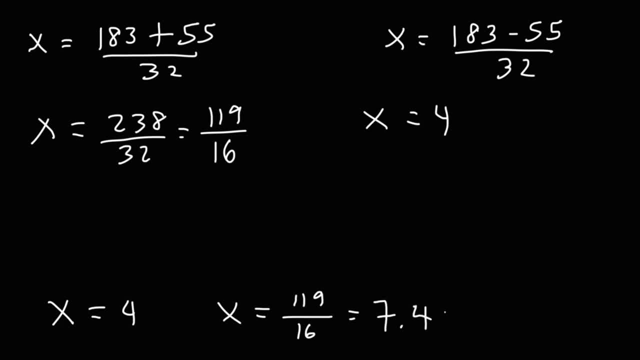 as a decimal, that is 7.43.. Now we need to check for extraneous solutions. We need to make sure that both answers, or even one of the answers, is correct. So let's go back to the original problem, where we had the square root of 4x plus 3,. 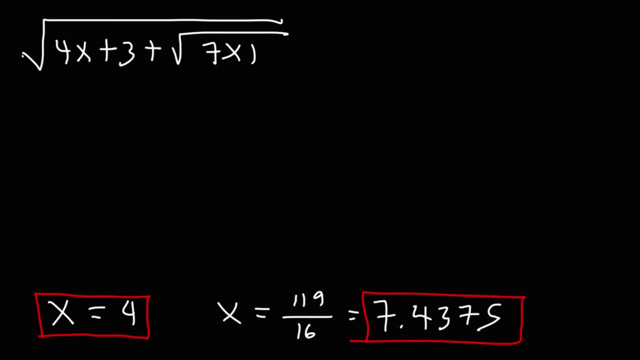 plus the square root of 7x plus 8, which equals 5.. So let's start with this, Let's see if that's going to work. So let's replace x with 4.. 4 times 4 is 16, and 16 plus 3 is 19.. 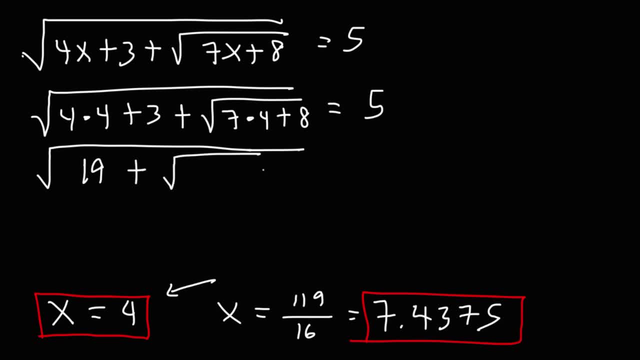 Inside the other radical, we have 7 times 4,, which is 28,, and 28 plus 8 is 36.. Now the square root of 36 is 6,, and 19 plus 6 is 25, and the square root of 25 is 5.. 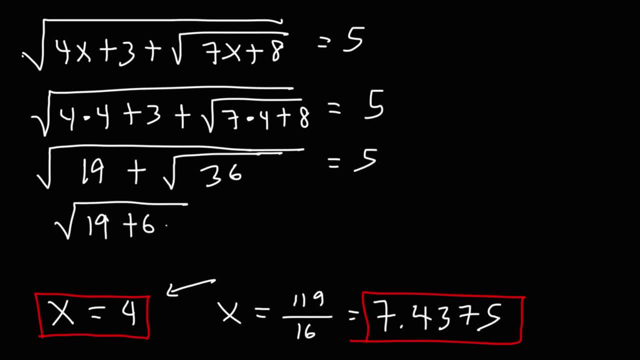 So this answer is correct: x does equal 4.. Now let's check the other answer. So we're going to have the square root of 4 times 119 over 16, plus 4, which is 16.. 29 plus 6.. 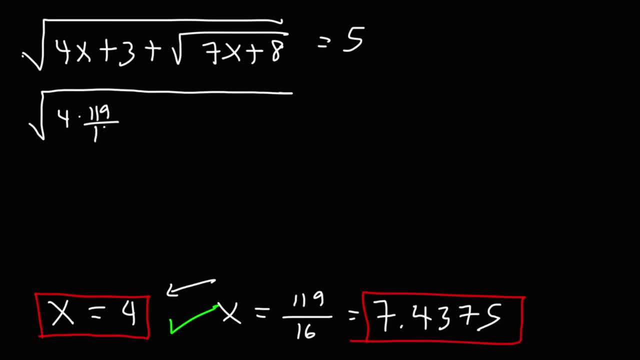 And the square root of 7 times 4 is 9.. That's 4.. So right off the bat we'll have 5.. 0.4x 3 plus the square root of 7 times 119 over 16 plus 8.. So I'm definitely going to use my calculator. 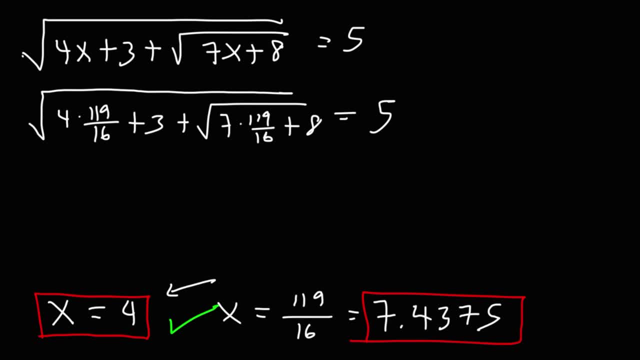 for this one, 7 times 119 over 16 plus 8, that's 60.0625.. Taking the square root of that, it gives us 31 over 4, which is 7.75.. Adding that to 3, that's going to be 10.75.. And then 16 divided by: 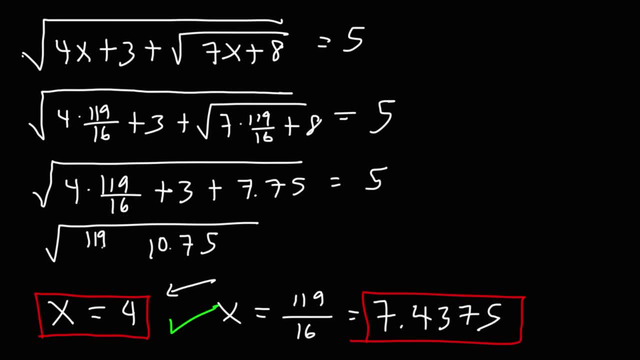 4 is 4.. So 4 times 119 over 16, that's just 119 over 4.. 119 divided by 4 as a decimal is 29.75.. Add that to 10.75, that gives you 40.5.. 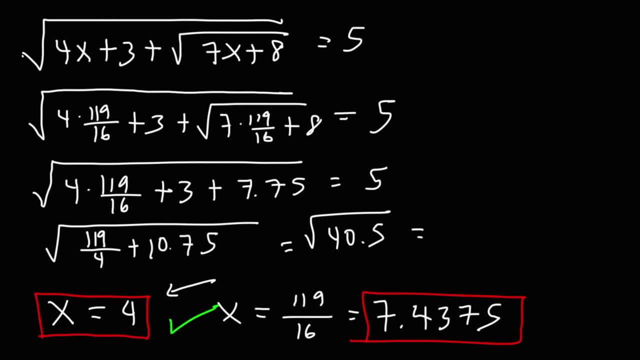 The square root of 40.5 is not 5.. In fact, it equals 6.36396 with some other numbers, And that doesn't equal 5.. So therefore, this solution doesn't work. So we only have one answer for this.